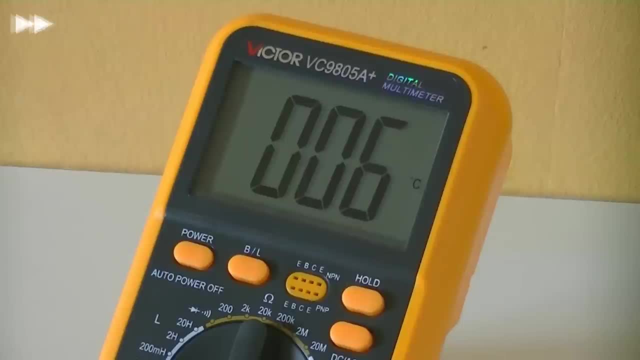 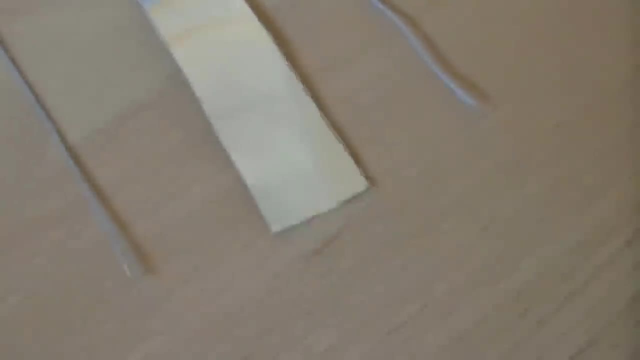 a difference of temperature by using electricity. It's called the Peltier effect. We are going to show you the Seebeck effect through a basic experiment. Practically speaking, it works with metal cobbles. We will join two metals and bring that junction to a certain temperature. 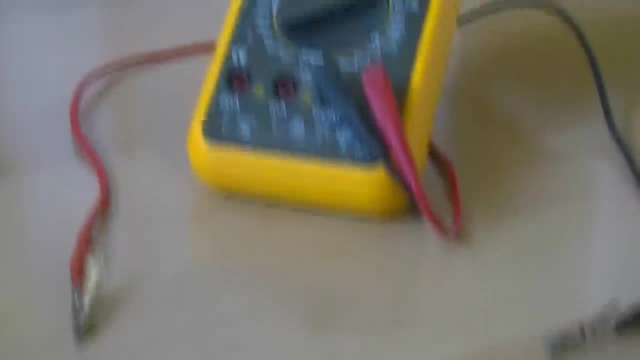 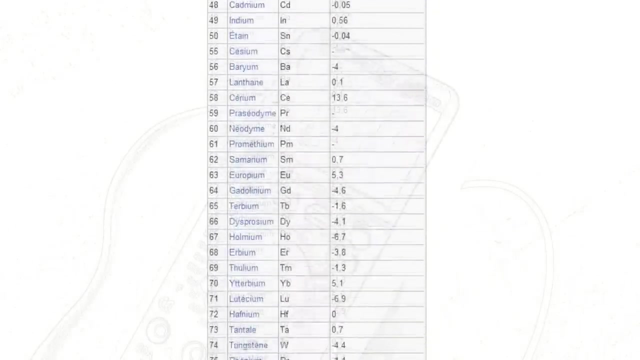 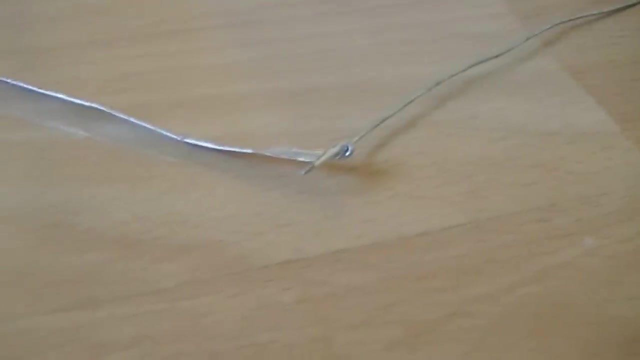 Then put a second identical junction to a different temperature. It's very simple, but it should create electricity. It should be pointed out that each metal has its own Seebeck coefficient and that the aluminium-iron couple is by far the most efficient one regarding common metals. 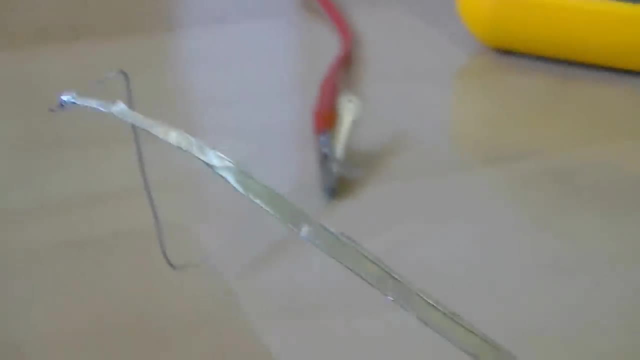 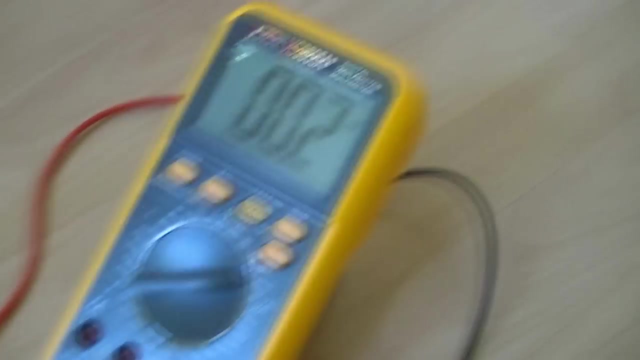 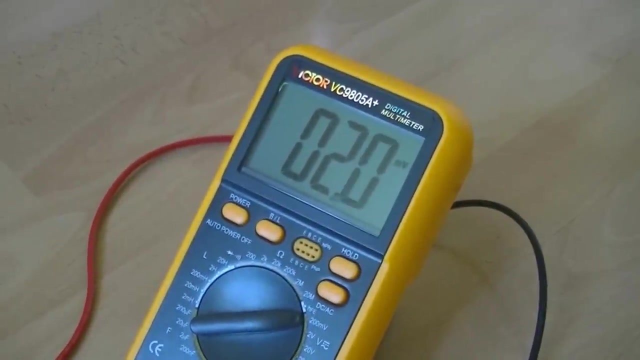 We've listed one of the junctions so we can heat it up with a flame Meanwhile. the other is going to stay at room temperature. Ok, it's hardly producing 3mV for a 20uA current only, but at least we've observed the effect. 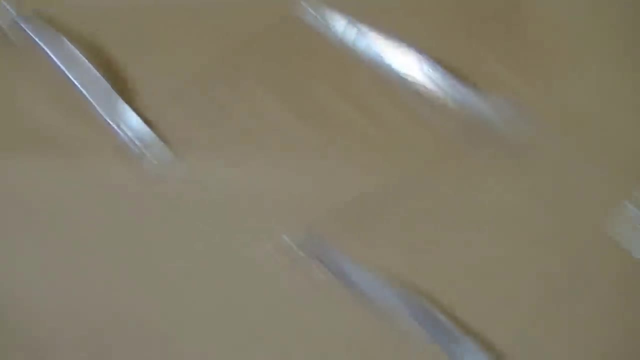 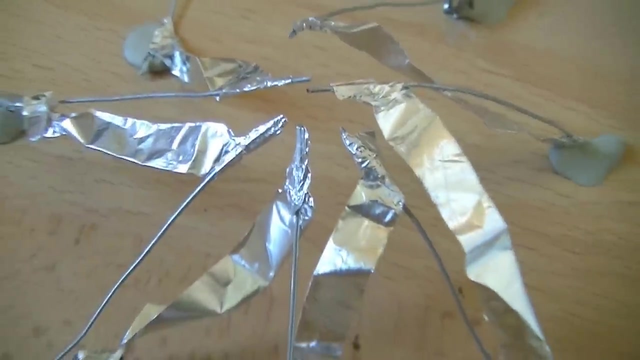 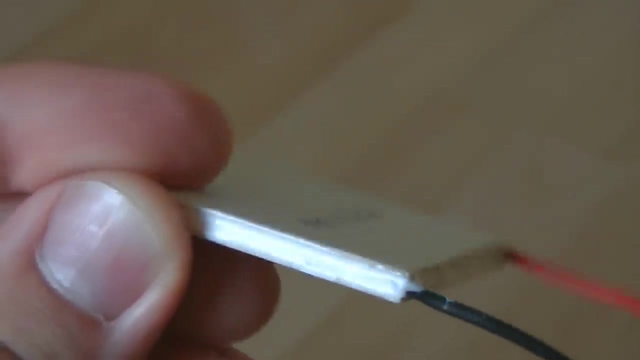 we were looking for. We can do much more by using a couple of junctions in series. They are placed alternately at hot and cold sources, But the production stays at about 10mV tops, making the power ridiculously low. Fortunately, we can do much better than that, thanks to manufacturer goods which gather 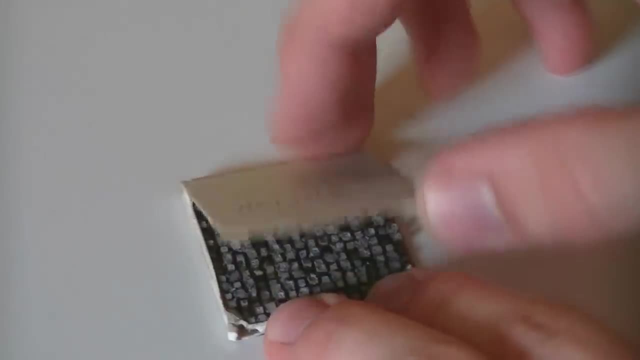 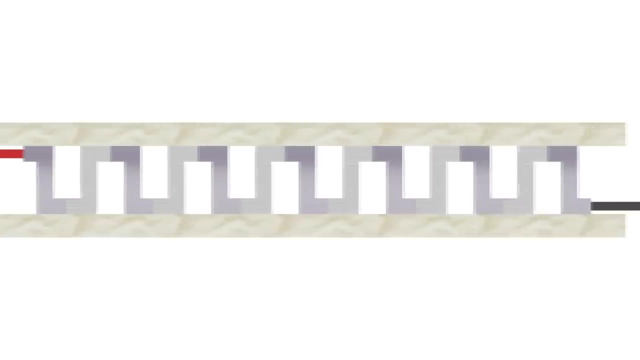 many junctions with specific metals. They are called Peltier modules. They can almost only be found in car electric coolers. They are used to produce cold from an electric current, But of course they are reversible. So let's start with the Peltier modules. 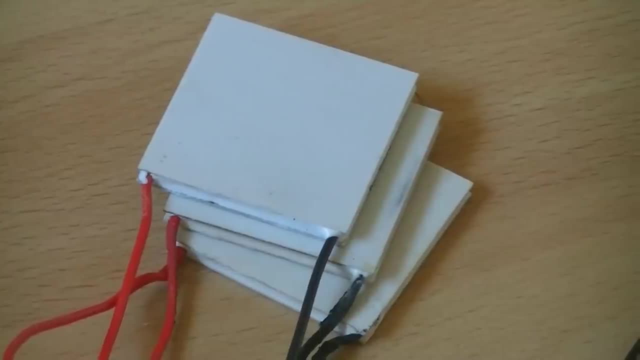 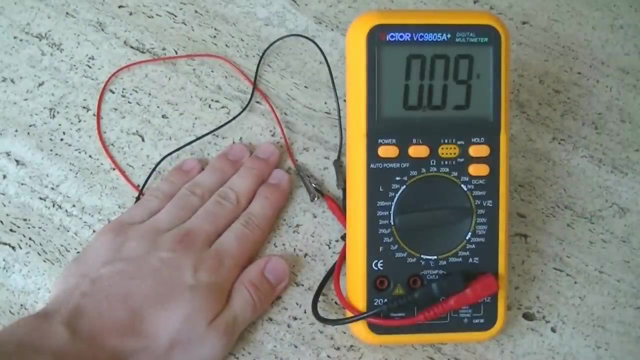 The Peltier modules are made of steel. They are made of steel. They are made of steel. We bought a few of those on eBay for about $13.. Let's see together what happened. I put my hand on one side of the Peltier module. The other one stays cold as it's pressed. 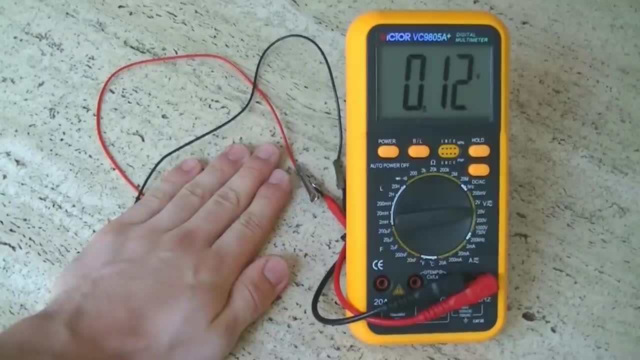 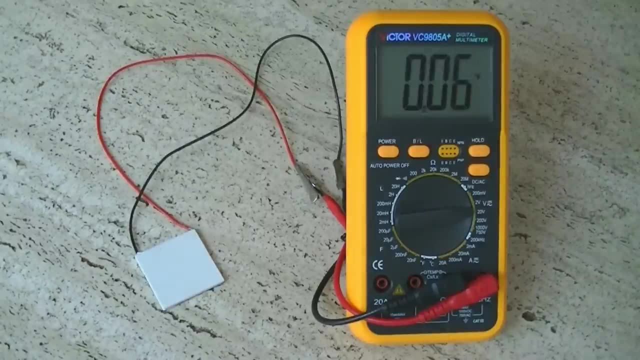 against the stone. We can already observe that more than 0.1V is produced with that temperature difference. We even managed to run a tiny motor with 4 modules in series. Now let's see what happened with the flame, The heat flow moving from the hot side to 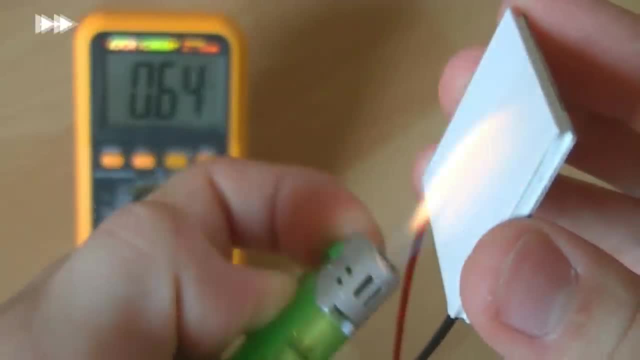 the cold one. make it work. The moment we stop heating the module, the heat flows from the hot side to the cold one. The moment we stop heating the module, the heat flows from the hot side to the cold one. The moment we stop heating the module, the heat flows from the hot side to the cold one. 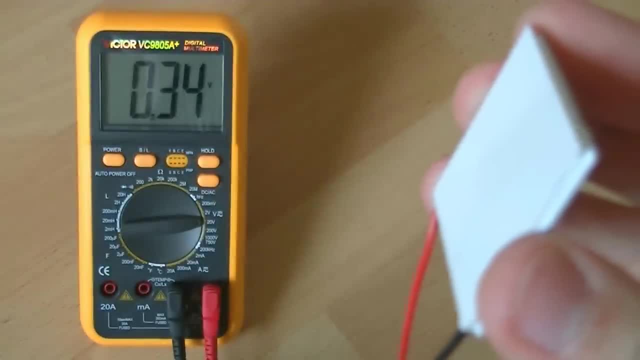 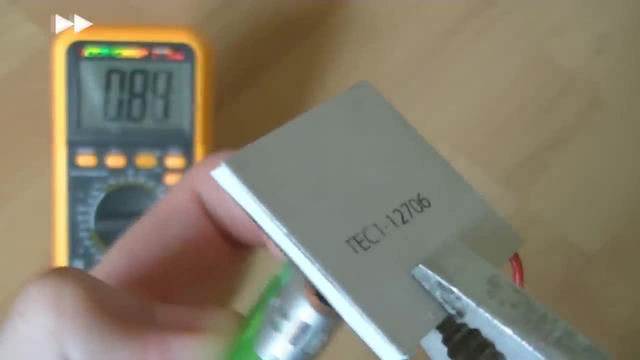 And in fact even more than 0.1V, the produced voltage decreases. We just saw that there needs to be some heat transferred from one side to another to produce something, But after a while the cold side becomes practically as warm as the hot one. From there the projection doesn't get any. 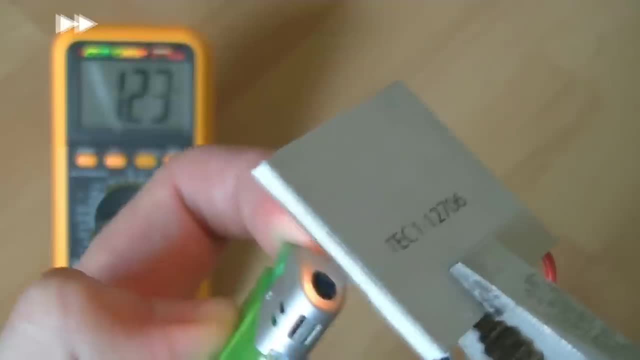 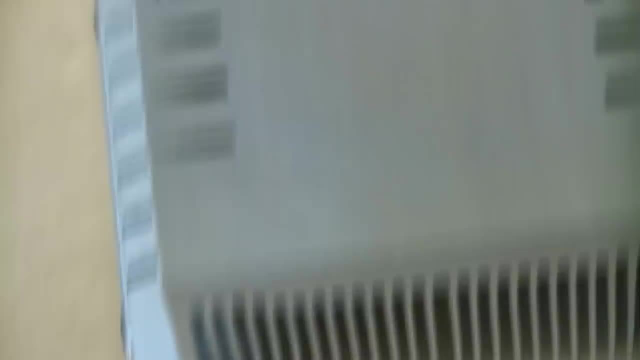 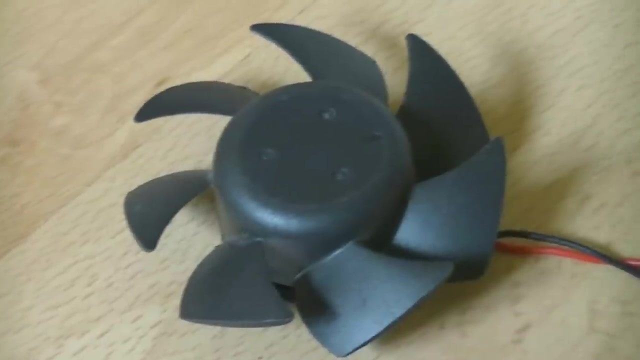 higher, We can clearly see that the voltage reaches the maximum point before decreasing gradually. To remedy this situation, we are going to use a big computer cooler, which would prevent the cold side from warming up As the radiator ended up getting hot himself. we've added a little fan. 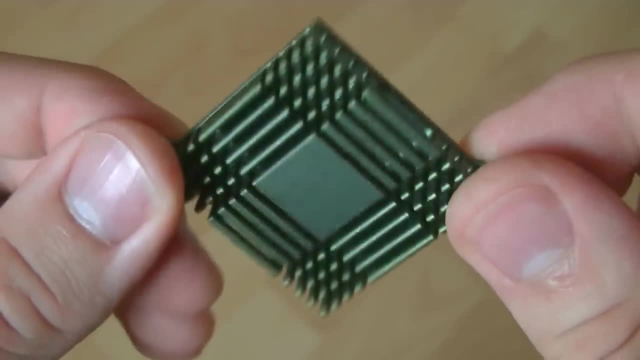 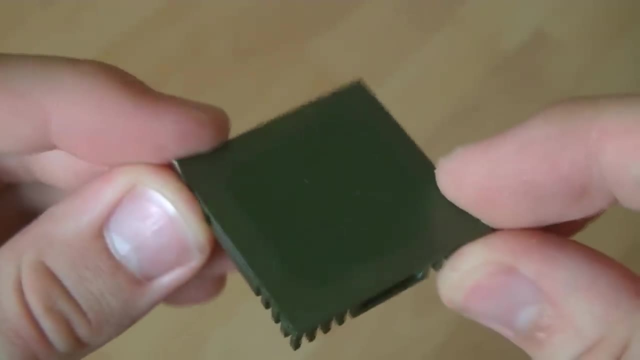 We are also going to use a little radiator on the hot side so that the flame's heat equally spreads on all the junctions. It may look insignificant, but it considerably increases the performances and prevents that kind of things from happening. BLEH. 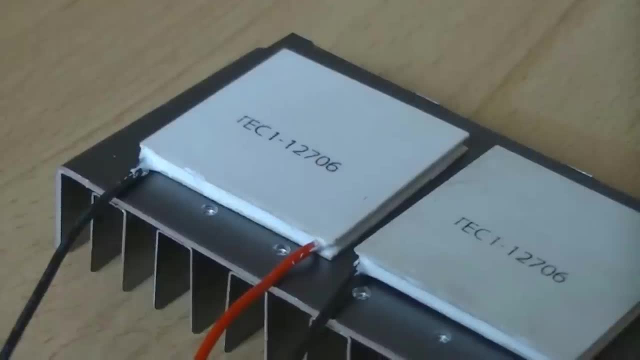 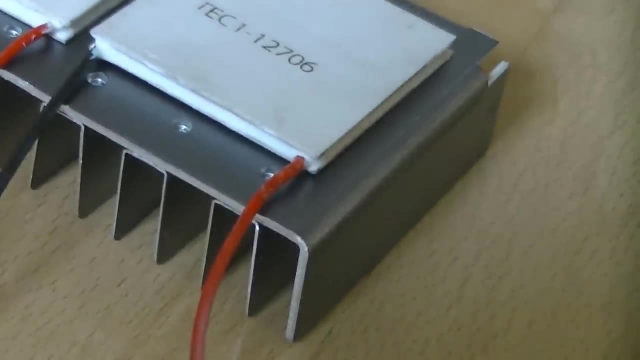 Contrary to one might think, to produce as much voltage as possible with a single flame it's better to use a single peltier module which can easily be heated at a very high temperature. If you put several modules, the power spreads. the temperature of each module decreases. 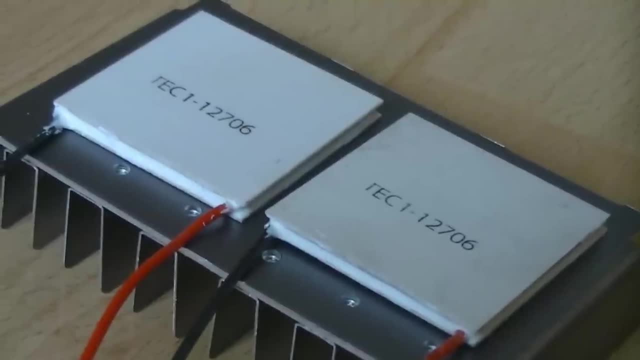 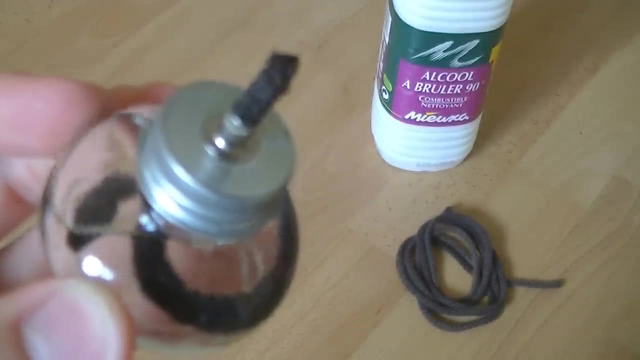 and it produces less. It's a consequence of the second law of thermodynamics. You can easily build a burner with no more than alcohol and a shoelace. We have everything we need now to make it work. let's see how it goes. 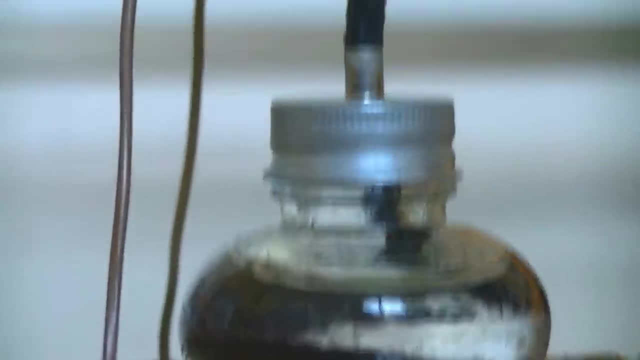 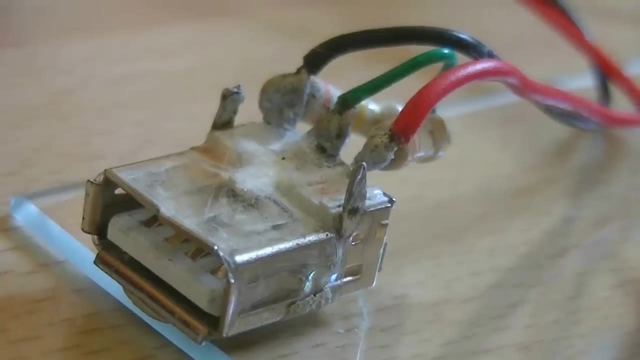 You can see this is the filter and here it's going through the vacuum. You can see it's in full mode and if you turn on that it's in full flat mode. It's nothing to worry about, It's just a clock. 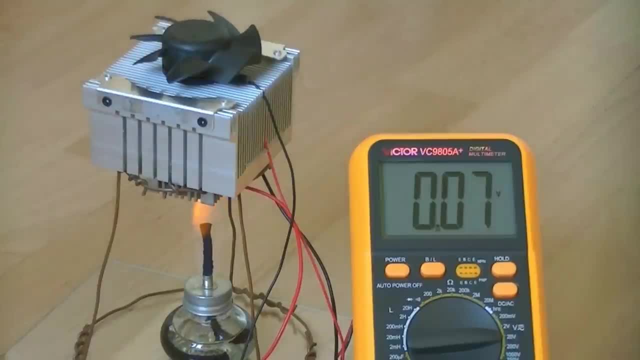 It works just fine. You can actually see. you can see it. You can see the west side. it moves. you can look at everywhere. You can actually see that it's in full mode, but here it's in full flat mode. 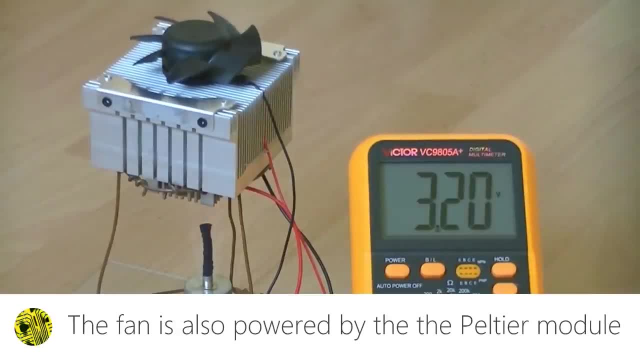 That's fine, Let's leave it there. Now we'll show you an example of how it works. We're going to build a house and a house. We're going to put a fence on the house. We're going to build a house. 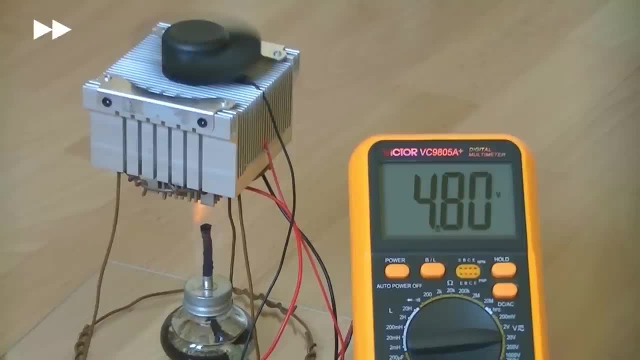 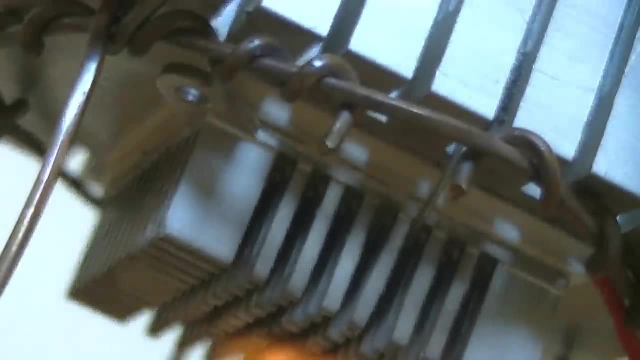 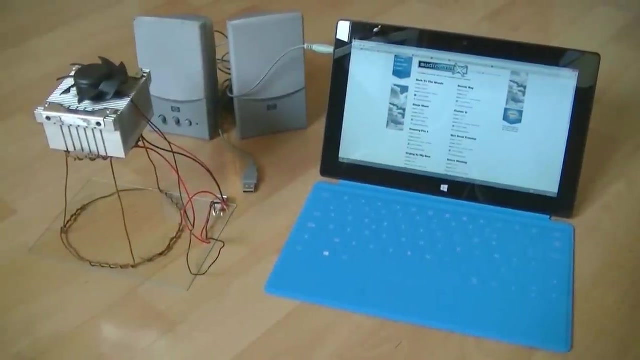 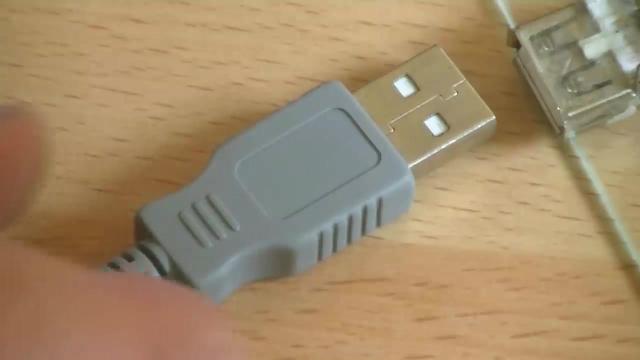 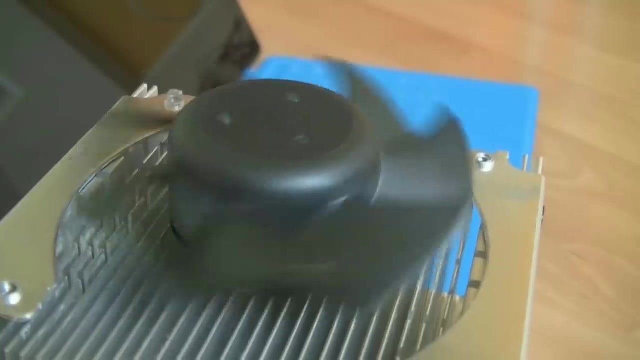 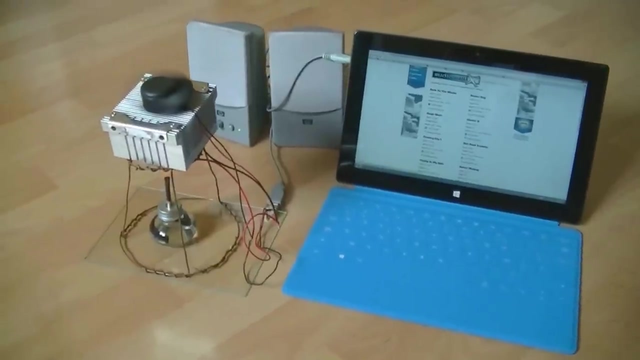 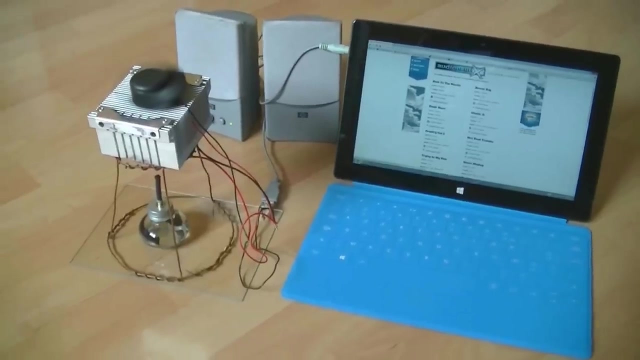 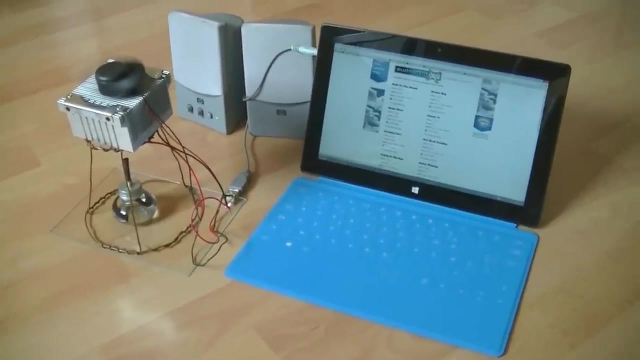 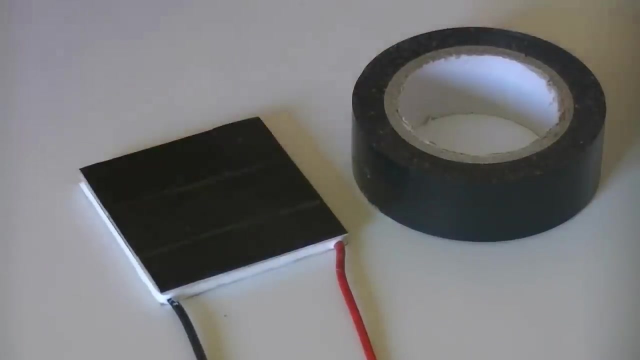 Here's a house. We're going to put a fence on the house. Here's a house. Let's go. Let's go a little further and see what we can get from the sense power To do that. we cover the side to be heated in black. 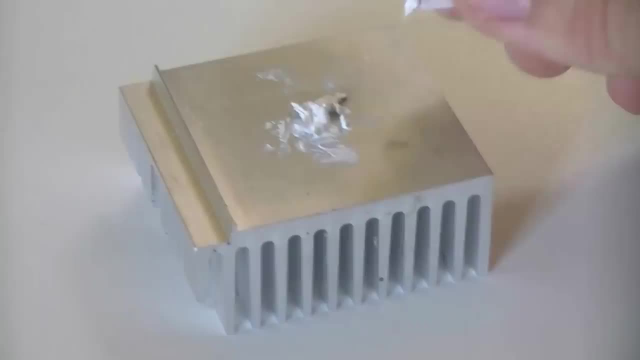 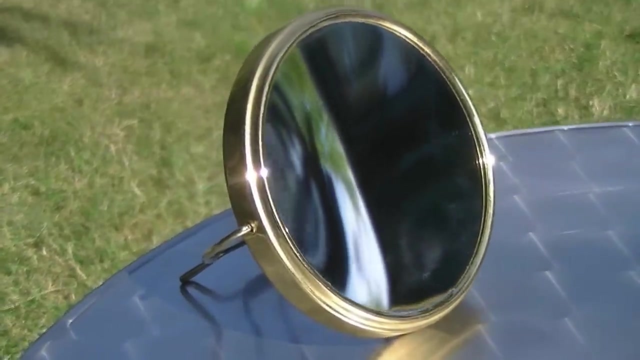 and put some of the heat on the other side. We use a radiator on the other side to dissipate heat, Some thermal paste to join the two sides and we are ready to go for the outside test In order to concentrate the rays of the sun on the module. 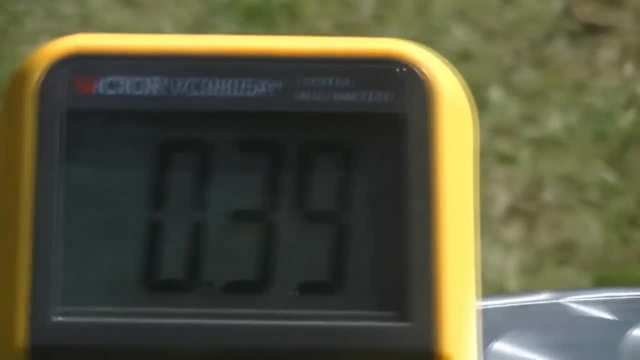 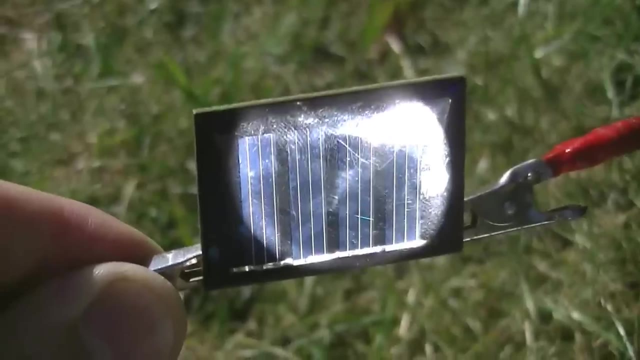 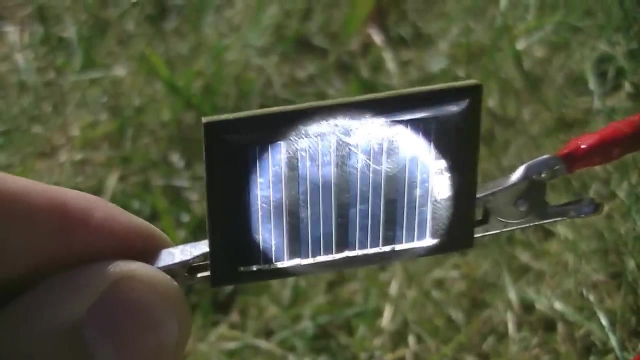 we use a parabolic mirror, We can see that we produce enough power to supply an electric motor. It works. but solar cells are far from being a poor second to Peltier modules. Indeed in our conditions a solar panel of the same size. 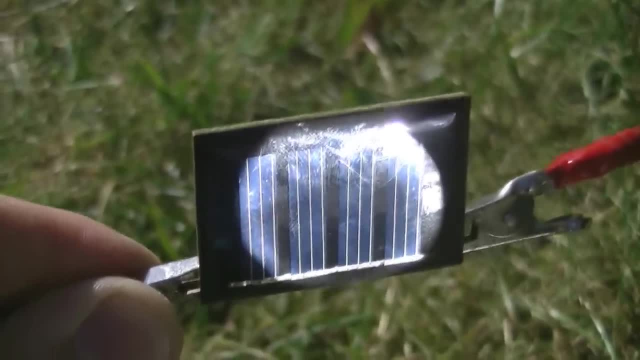 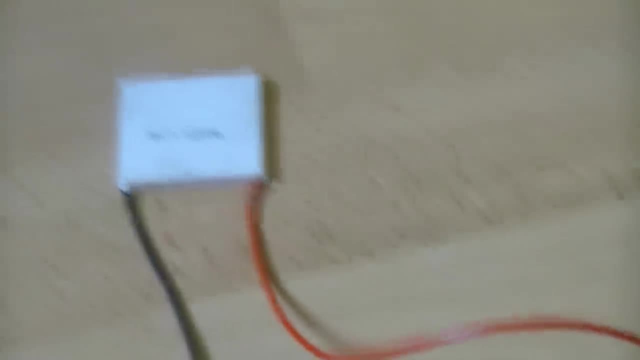 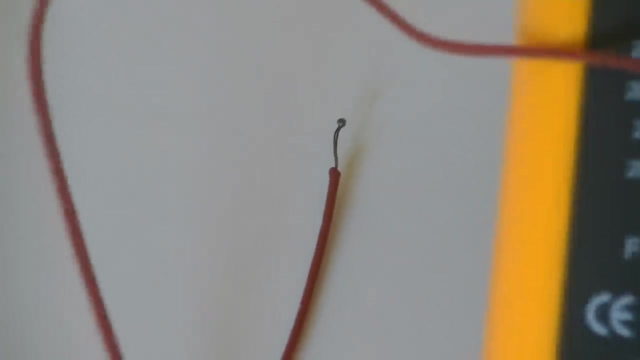 produces 18 times more than a Peltier module. Now we are going to conduct some experiments concerning the Peltier effect. We are going to send some electric current into a module. We are then going to use a digital thermometer. By the way, most top-observing thermometers works with metal couples. 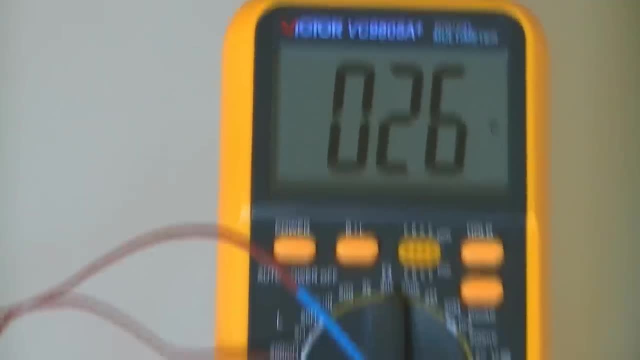 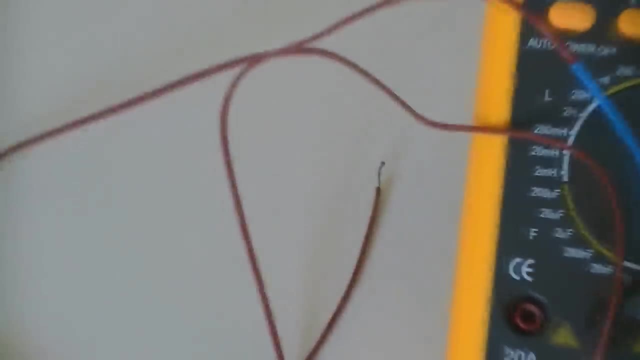 We talk about thermocouples. The more the junction warms up, the more voltage is produced. It's precisely the Seebeck effect we talked about at the beginning of the video, which is involved here, to measure temperature Depending on the current direction. 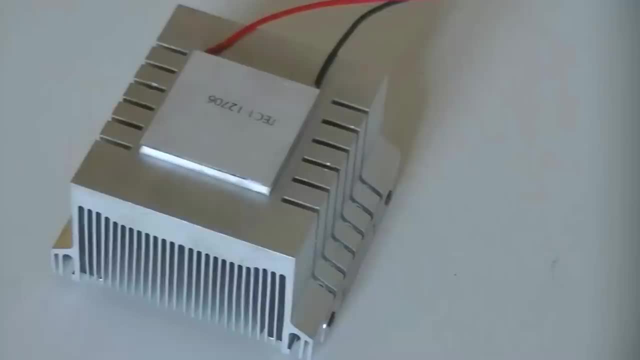 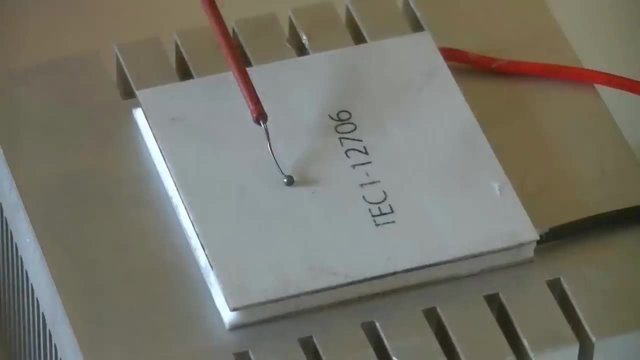 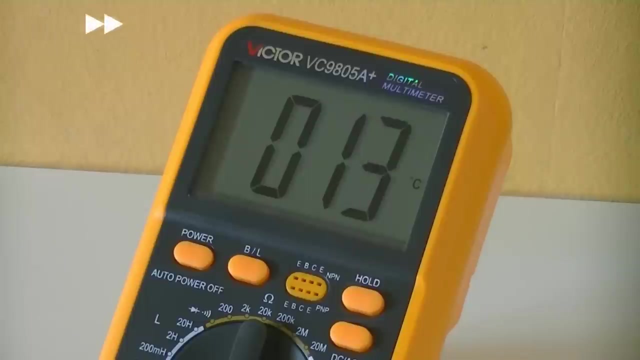 one of the sides should heat up and the other should cool down. We also put the hot side on a radiator, which allows the cold side to be even colder. It works. the temperature gradually decreases and reaches its limit around 4°C. 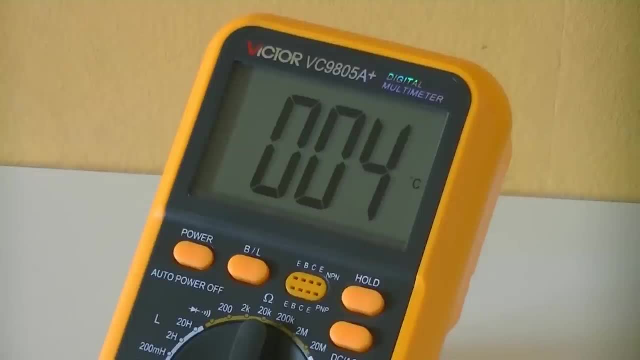 In fact, that limit corresponds with the moment when the heat of the module decreases. In fact, that limit corresponds with the moment when the heat of the module decreases. In fact, that limit corresponds with the moment when the heat of the module decreases.